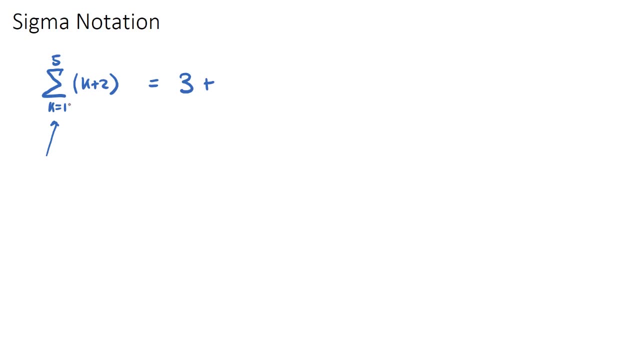 by all of the integers. So you go to k equals two. So if k did equal two you'd sub the two in: Two plus two is four, So four will be our term and then we need to sum again: K equals three. 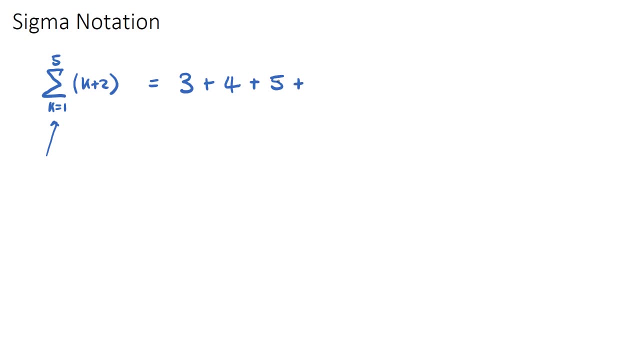 Three plus two is five. Then we need to sum again: K equals four. Four plus two is six. Now when do we stop? Well, we stop when k reaches this top number, which, in this case, is five. So this will be the last one. If k is now reached, we're going to have a five. So we're going to have a five. 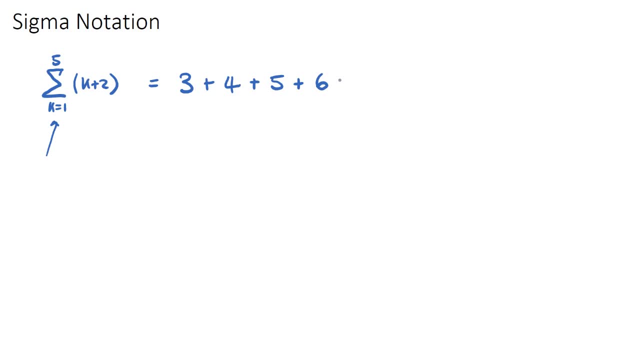 If k reaches the top number, five five plus two is seven. So this here actually just means three plus four plus five plus six plus seven. It's this equation if we sub in the starting value and we keep going up to the end value. So if we just add this up we're going to get seven plus five is. 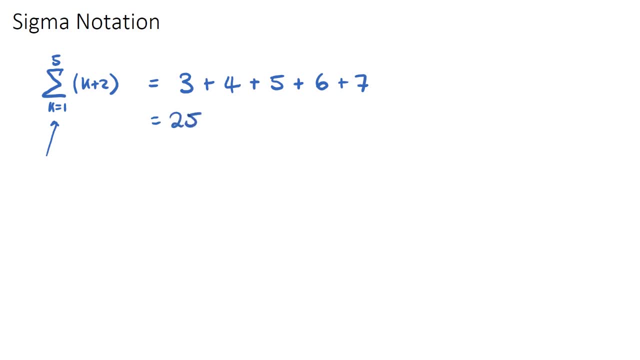 twelve and eighteen, and then twenty-five. Okay, so this is an example of what sigma notation is. If we have something like this, this is the more compact form. Okay, I'll do another example. Let's just say we have: let's go with a sigma, Let's go k equals. 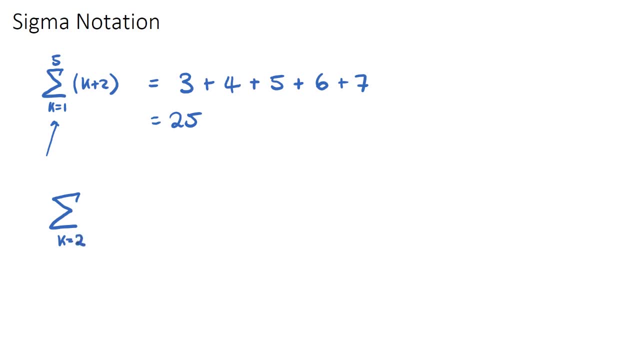 and we're going to start now a little bit different. I'm going to start at two and go up to five. This can be any number here- and I'm going to have one over two to the k. Okay, let's use what we did up here. This means we start with our first value and k equals two, and 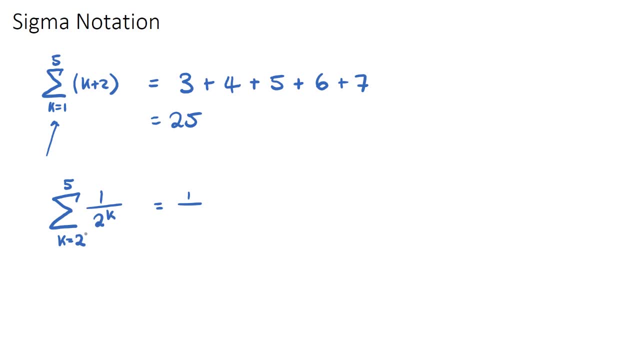 then we add that in, So we're going to get one over two to the power of two, So one over two squared, and then sum and then we have k equals three. It'll be one over two to the power of now. k is three. 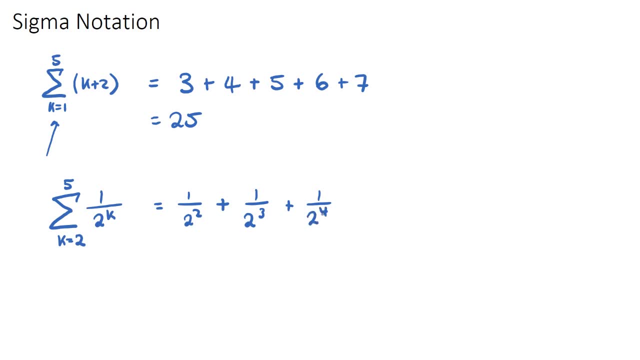 plus one over two to the four, and we stop once. k is our top number. So plus one over two to the five. Now we can work this out. This is one on four plus one on eight. Plus one on two to the four is 16 plus one on 32.. And I think you get the message here. We could 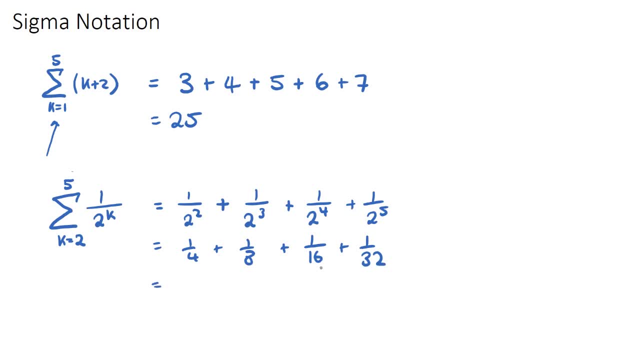 all get a common denominator. I will do it. This is still going to be one on 32.. Our common denominator here will be 32.. So we'll have two, 32,. this will be four, and 32,. this would be eight. And then eight plus four is 12, plus two is 14,. 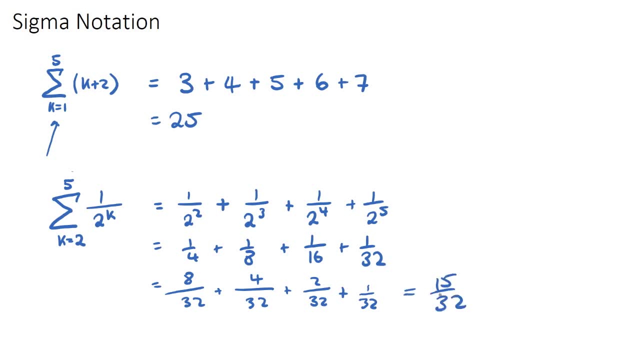 plus one is 15.. So this has a value of this. So in IB questions they do sometimes try and link sigma notation to arithmetic and geometric series questions, because think about an arithmetic and geometric series. It's when we're summing up an amount of terms and they might say: 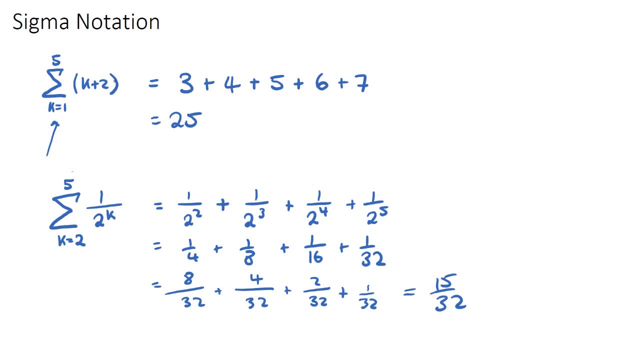 oh, I want you to find the sum of the first five terms And instead of asking that they might actually write it in this format- And this is where sometimes students who struggle to link the two topics- they'll look at this and go: oh, what's this Greek symbol here? 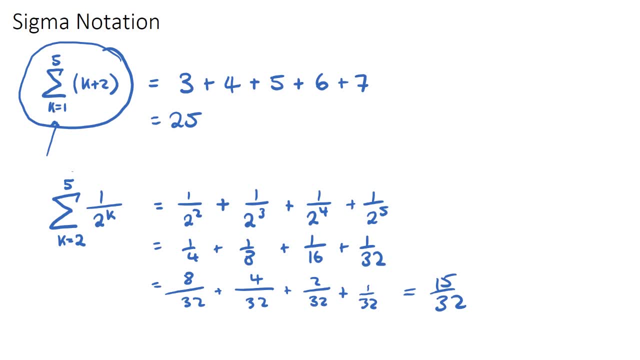 And I haven't learned this before, but this is actually just saying it's the sum of if we sub in our first term all the way up to our fifth term, and we're going to actually just get the sum of the first five terms. So these questions are actually just usually an arithmetic or a. 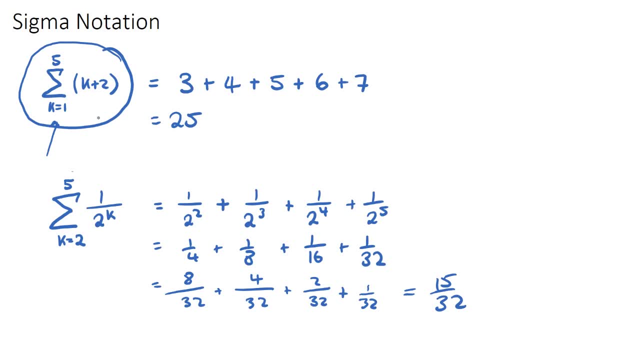 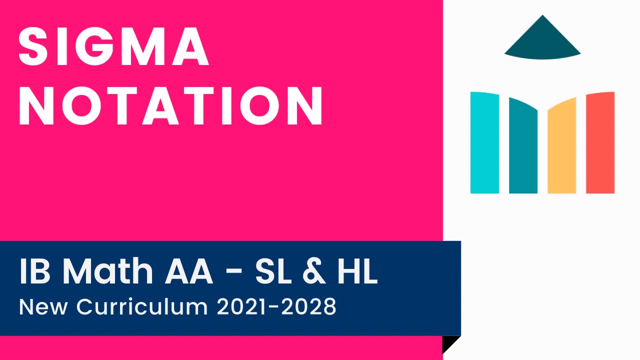 geometric series question. Okay, so that's just a brief introduction to what sigma notation looks like. Thank you.